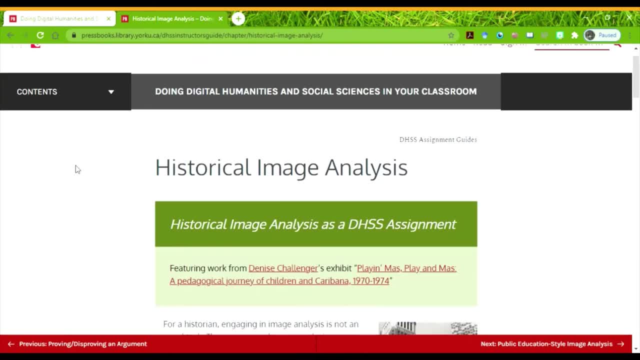 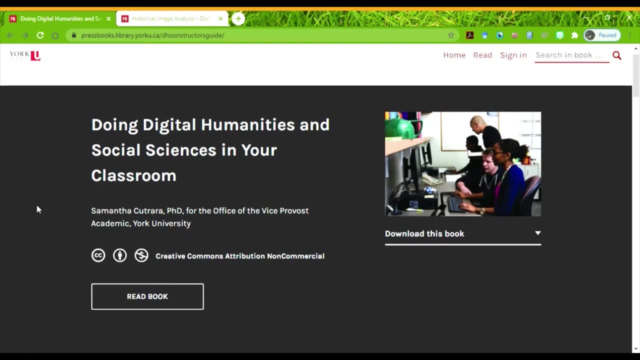 but I'm going to challenge that a little bit more. Before that, though, I just want to remind you that this activity guide, as well as all the activity guides, can be found in this ebook, this OER, which is an open educational resource, where I talk about the theory behind digital humanities. 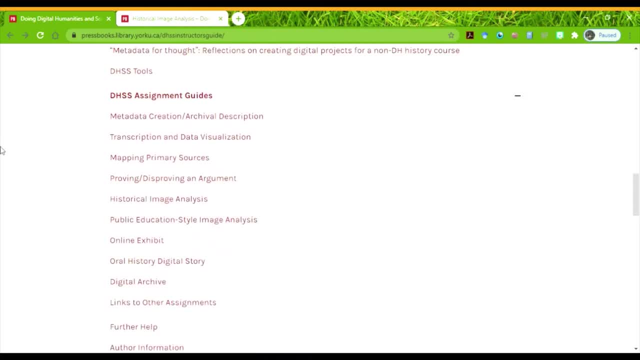 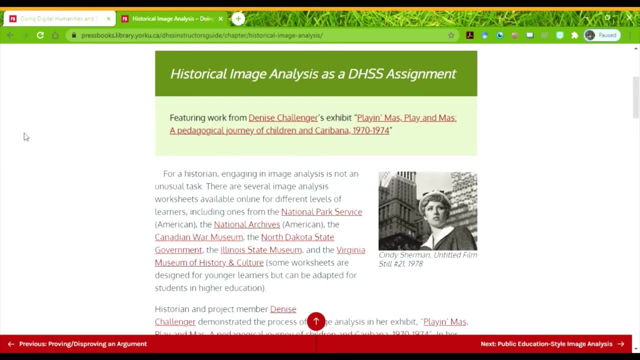 the practice and the assignment guides- And this is for novices in digital humanities- by someone like myself who's a novice- as well as the students that we did this work with- Although actually Denise knew more about it than I did, but we did some really interesting. 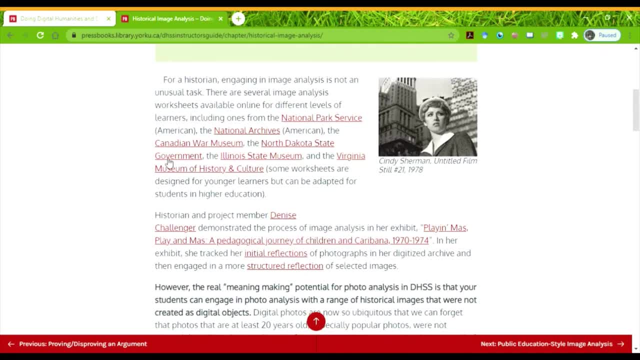 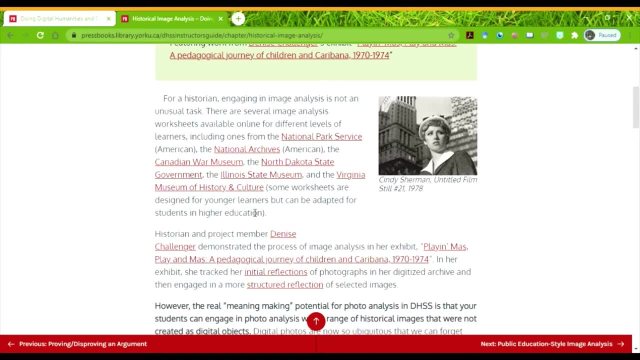 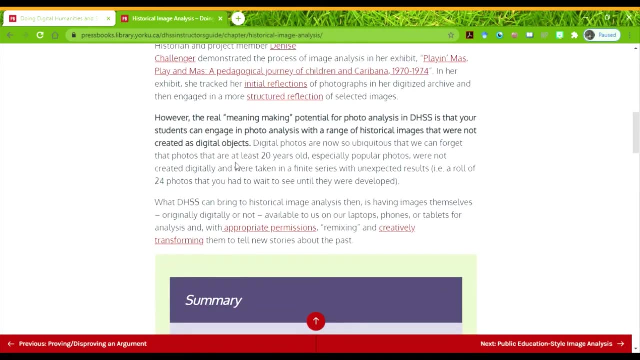 work that was able to complicate her understanding, which was really fantastic. So, yes, you can find a lot of Stuff online about analyzing historical photographs. We do not want to replicate this work, but instead I really want to challenge you to. 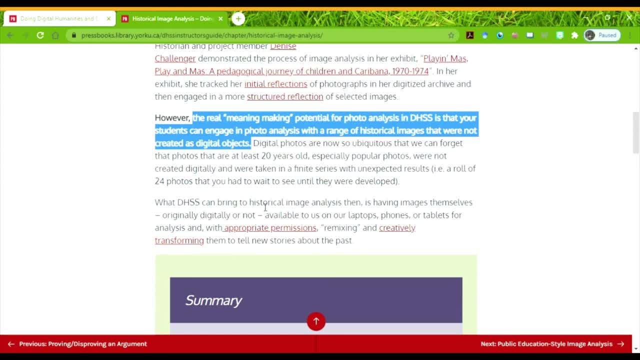 say that the real meaning making for photo analysis in digital humanities is that the students can engage with materials that were not created as digital. So what does it mean when students had to wait, like you know, a week to have their 24 roll photo? 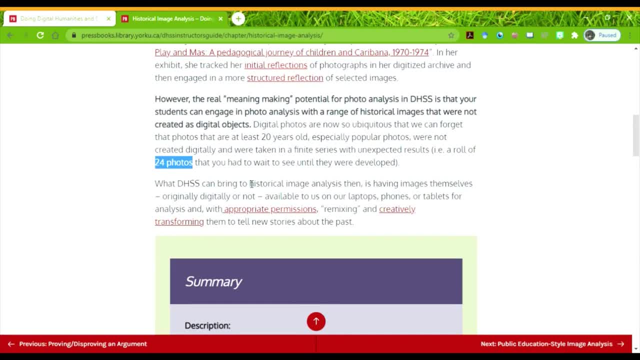 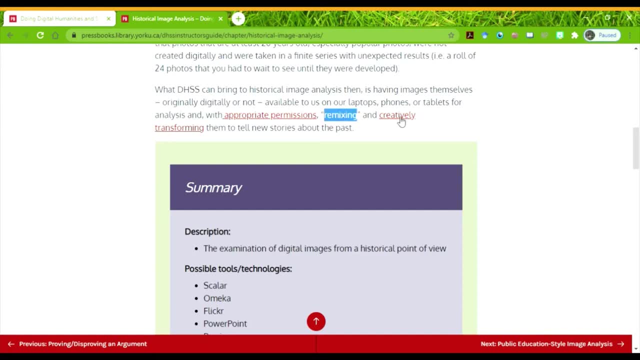 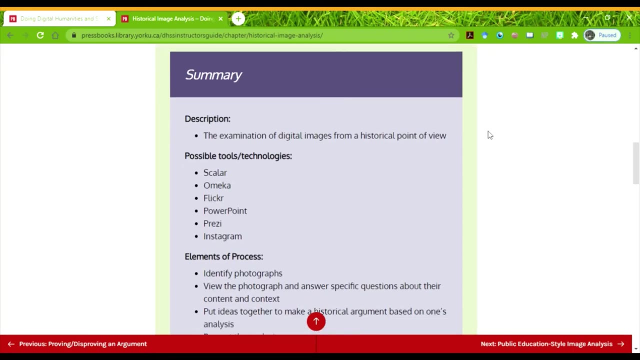 Um, uh, taken. What does it mean when you can't take a hundred photographs in a second? So get students to be able to think about these materials and Remix them creatively. transform these stories through their analysis to tell different stories about the past. 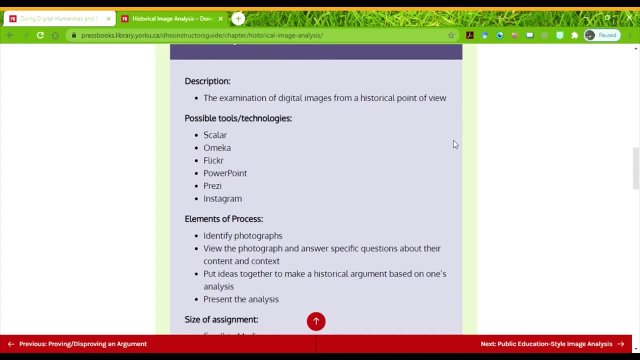 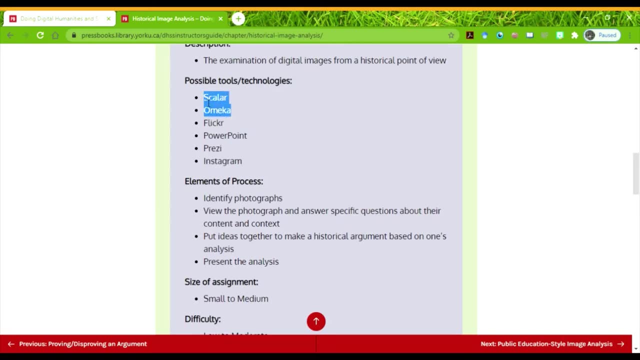 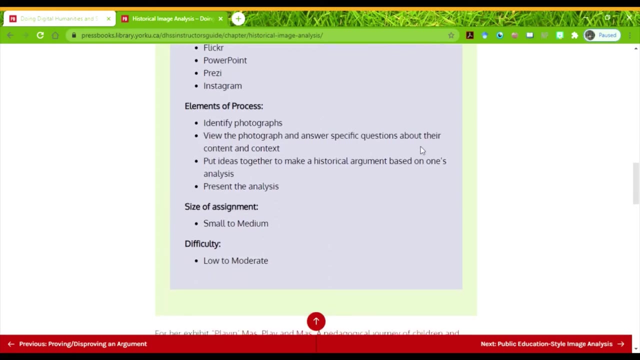 So it's an examination of digital images from a historical point of view. You can use PowerPoint, you can use Instagram, you can use Prezi and Flickr, but you can also use these online um exhibit tools, identify photographs, view the photograph and answer specific questions, but then put those. 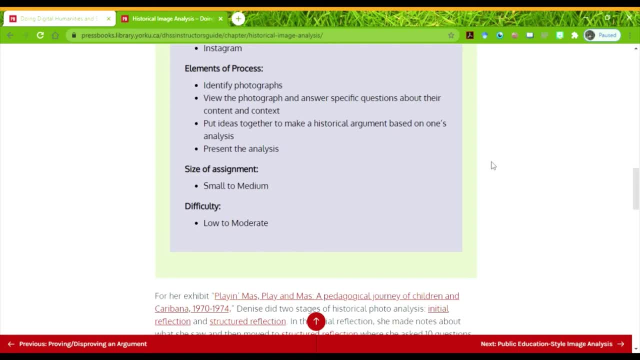 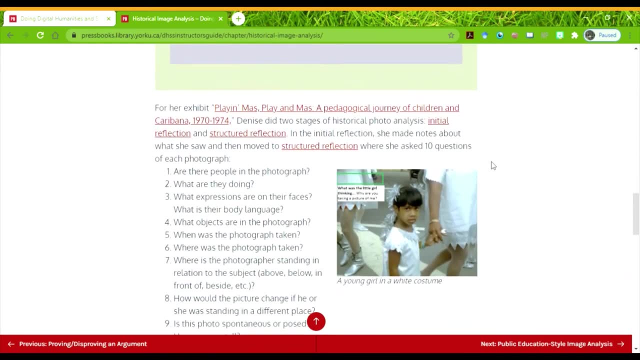 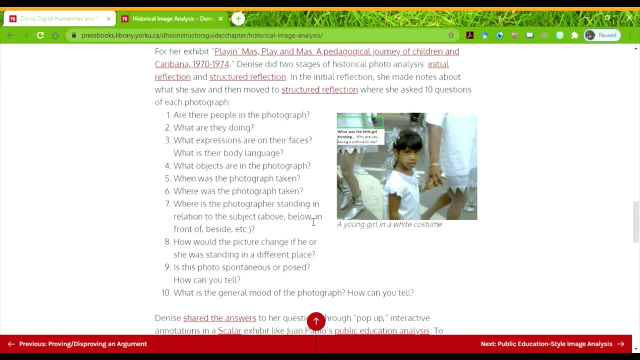 ideas together to make a historical argument based on the analysis and present that analysis. That brings us to a new element. So Denise looked at photographs from Carabana in 1970 to 1974, and she asked 10 questions about each photograph. These are fantastic questions. to start with,